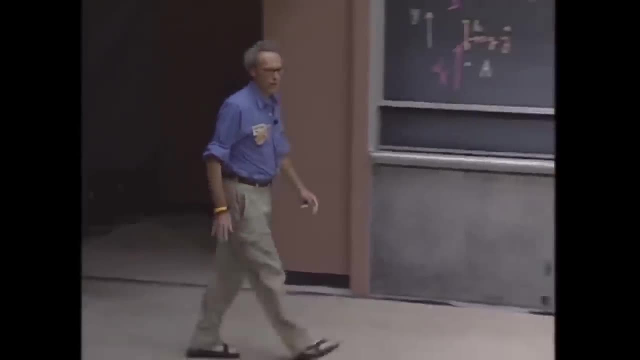 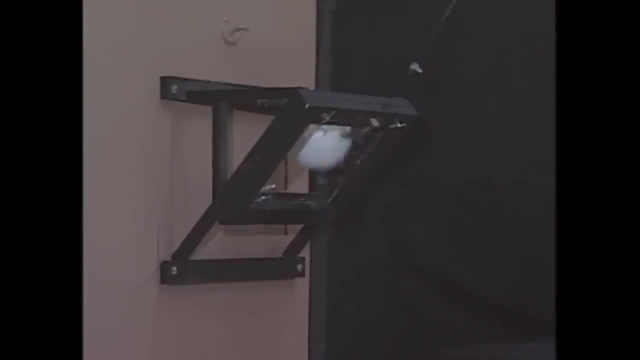 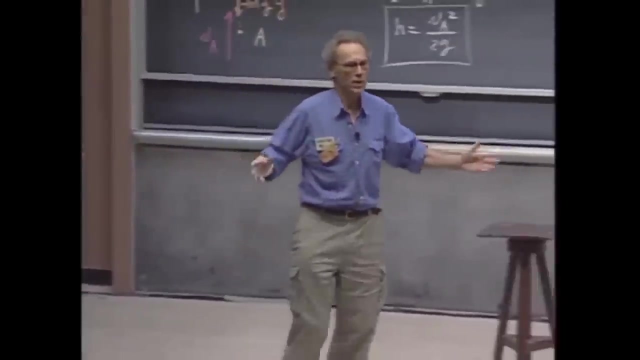 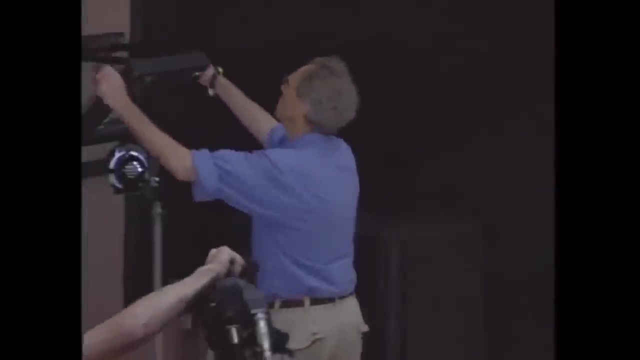 And that way you can demolish a building. You just let it hit and it breaks a building And that's the whole idea of wrecking. So you're using, then, the conversion of gravitational potential energy to kinetic energy. Now, I am such a strong believer of the conservation. 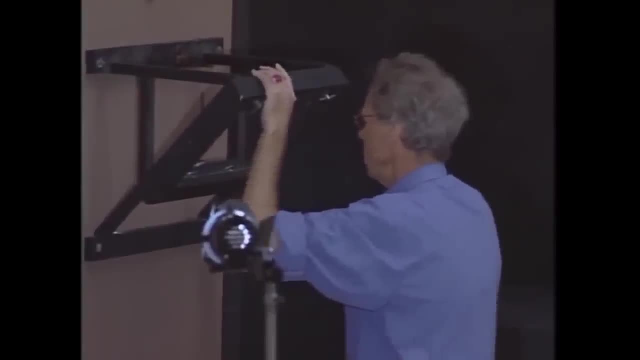 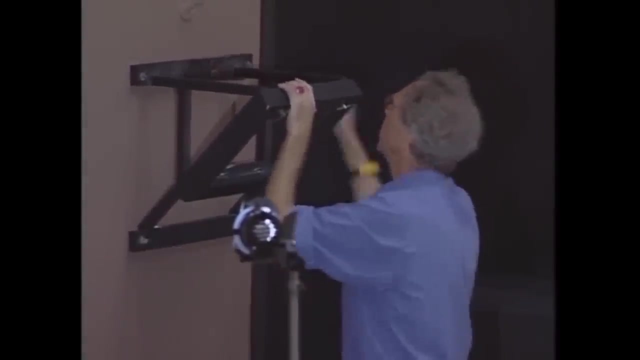 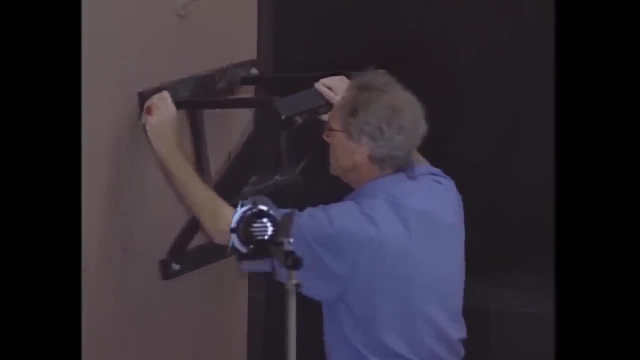 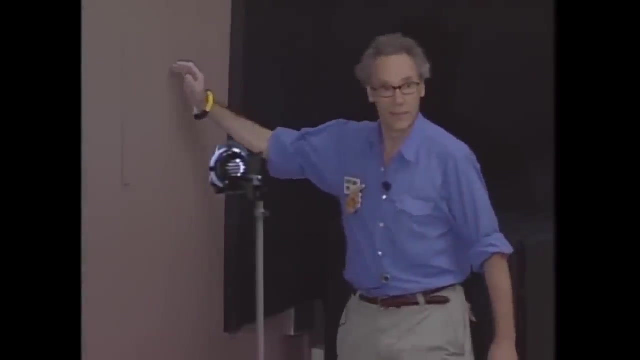 of mechanical energy that I am willing to put my life on the line. If I release that bob from a certain height, then that bob can never come back to a point where the height is any larger. If I release it from this height and it swings. 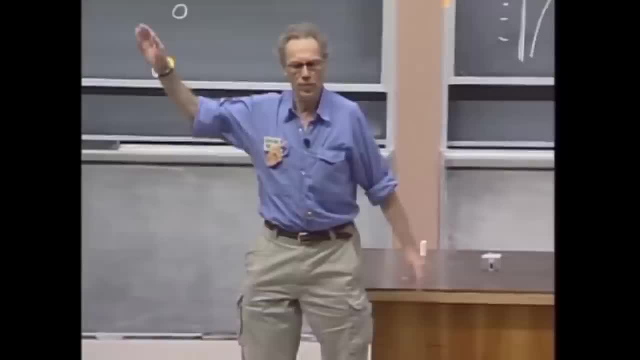 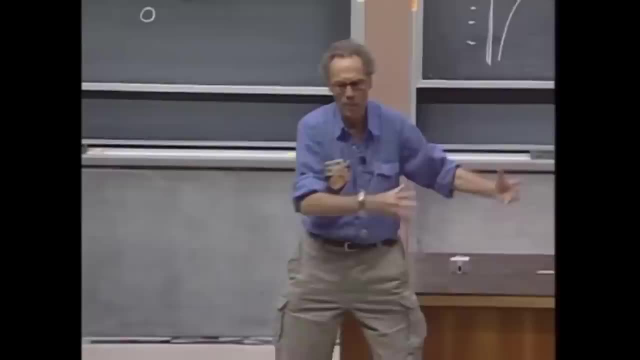 then when it reaches here, it could not be higher. There is a conversion from gravitational potential energy to kinetic energy, back to gravitational potential energy, and it will come to a stop here And when it swings back it should not be able to reach any higher, provided that I. 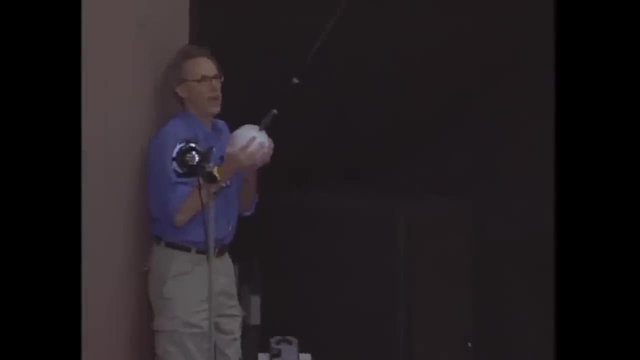 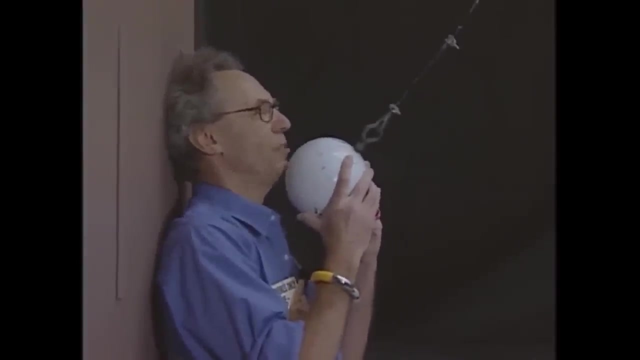 do not give this object an initial speed. when I stand here, I trust the conservation of mechanical energy for a hundred percent. I may not trust the conservation of mechanical energy for a hundred percent. I trust myself, I'm going to release this object and I hope. 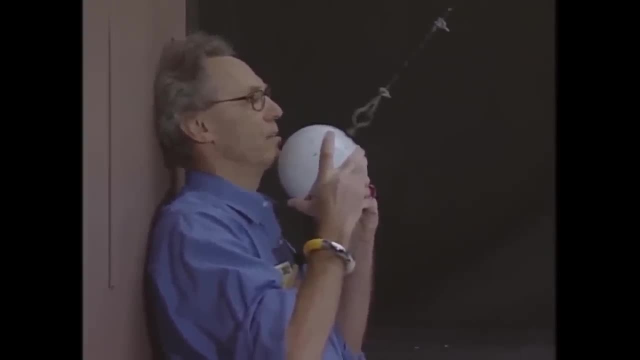 I will be able to do it at zero speed so that when it comes back it may touch my chin, but it may not crush my chin. I want you to be extremely quiet, because this is no joke If I don't succeed in giving it zero speed. 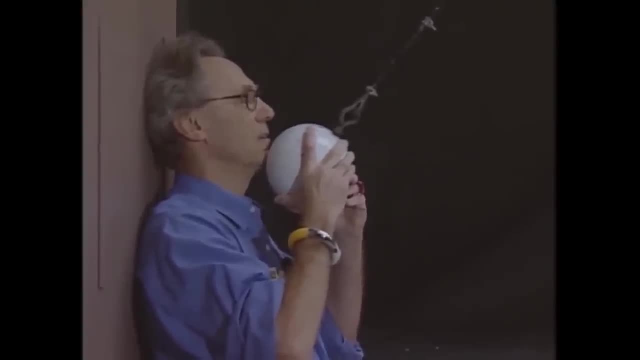 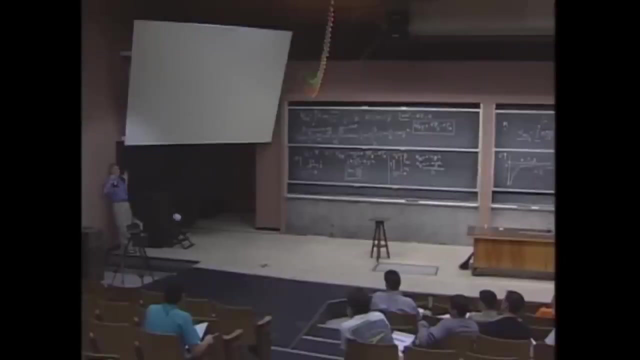 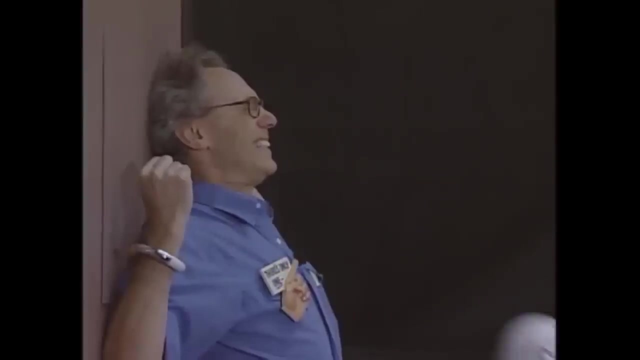 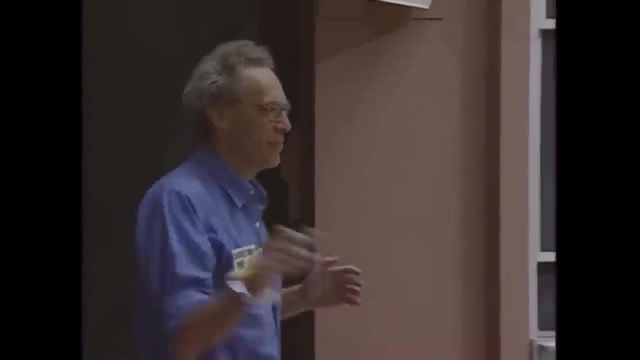 then this will be my last lecture. I will close my eyes. I don't want to see this, So please be very quiet. I almost didn't sleep all night. Three, two, one, zero. Physics works and I'm still alive.